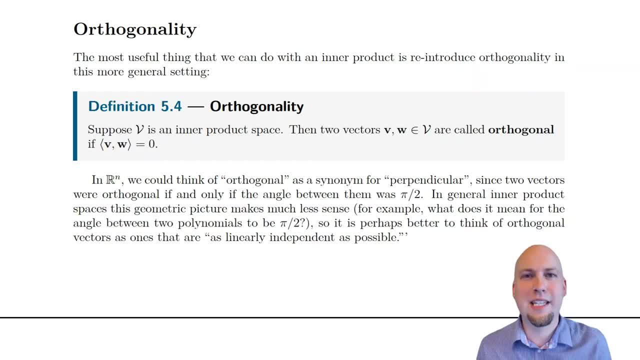 Hey folks, my name is Nathan Johnston and welcome to lecture 20 of Advanced Linear Algebra. Today we're going to talk all about orthogonality, which is something you learned about back in introductory linear algebra. Remember back then what orthogonality meant, was that two? 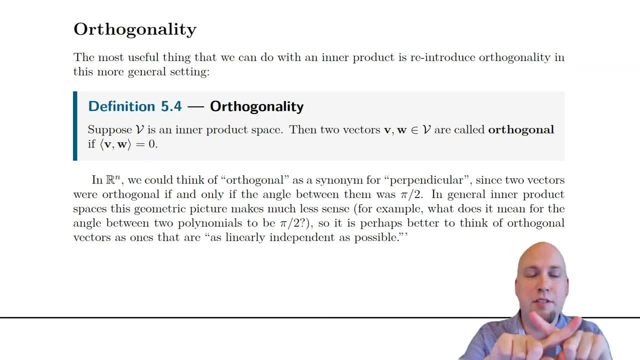 vectors were perpendicular to each other. The angle between them was pi over 2, or 90 degrees, And the way that you checked orthogonality was you computed the dot product between the two vectors. If that dot product equaled zero, they were orthogonal, And if it equaled anything, 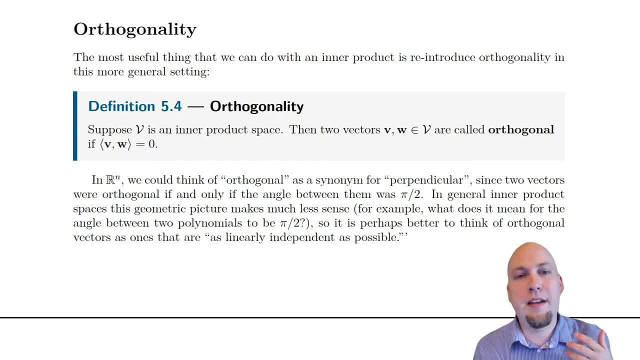 else they were not orthogonal. Well, now that we have inner products to work with as a generalization of the dot product, we can do the same sort of thing in arbitrary vector spaces. We can talk about orthogonality in arbitrary vector spaces just via this idea. 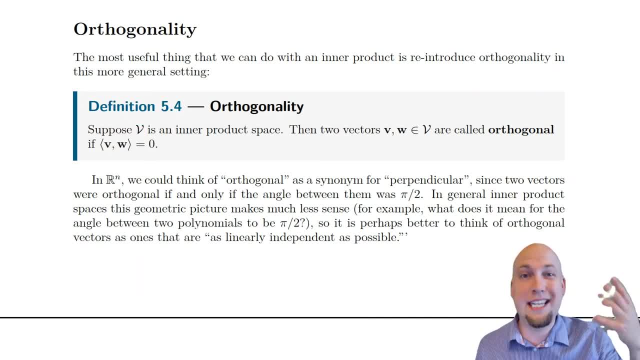 that the inner product now instead of the dot product, equals zero. So this is our starting point for this lecture: Orthogonality in any old inner product space, so in other words in any vector space with an inner product, equals zero. So this is our starting point. 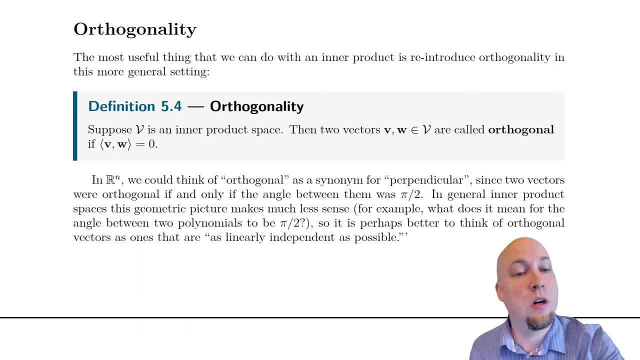 for dislocation in an entire vector space. What thatijo knows is that Chevy has established innovating Projektij ό�- whether or not this freaked outcja- of two 的or or, and we say that this is only inINTERPRODUCT. what that means, we say, is that two vectors are. 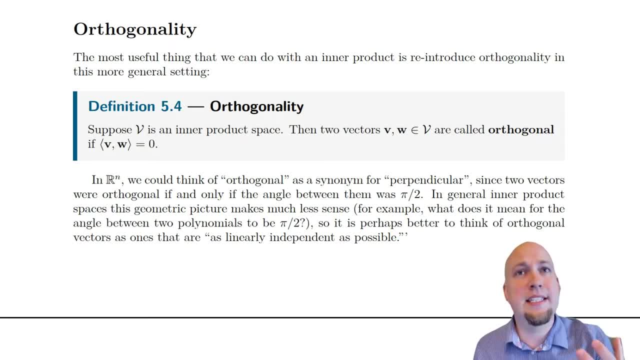 orthogonal if their interproduct equals zero And again. so the idea behind all of this, the intuition in INTUITION, is as it was back in RN, back when we were doing dot products: If vectors are orthogonal to each other, that sort of means they're in as independent as 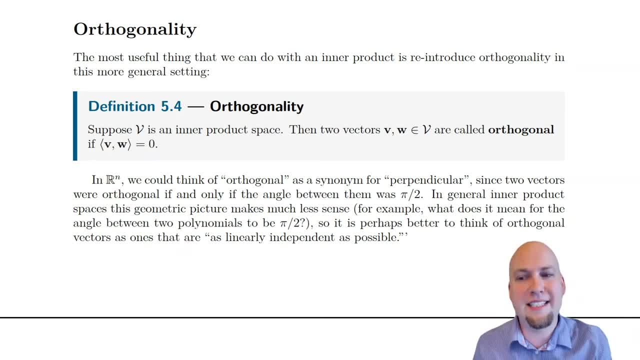 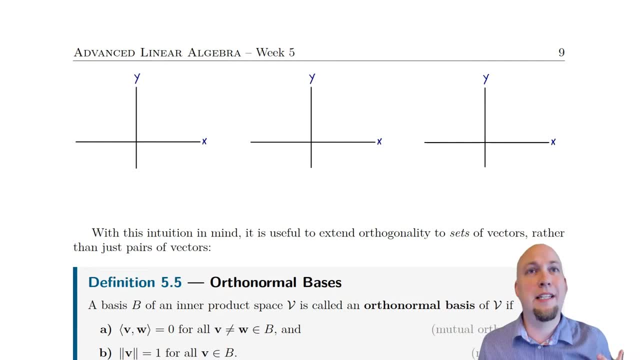 possible. in a sense, They are pointing as far away from each other as they can. OK, so let's draw a picture here to try to pin down this intuition. All right, first off, let's talk about linear nasties. Well, the sliding angle aroundródian is level 2p 독, covering rX and already that foretaken. 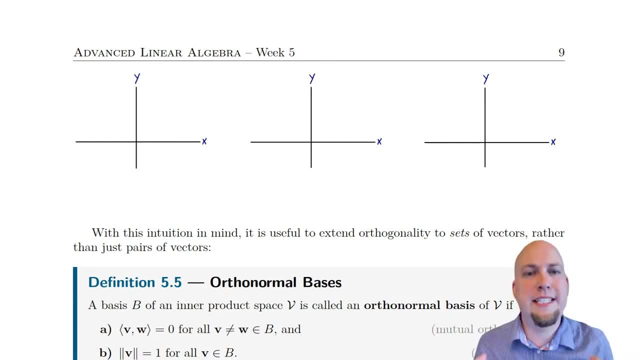 dependence. what that means geometrically? well, linear dependence just means that one of the vectors is a linear combination of the others, which, if you have two vectors, for example, means that they both point along the same line. right, they're in the span of each other. okay, so that's. 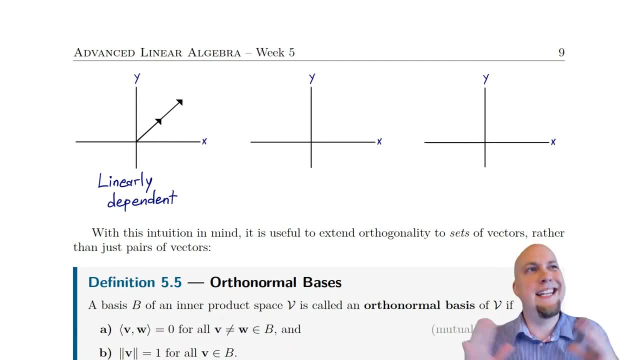 our linearly dependent picture, our linearly independent picture, just means: well, not that, it means they're, they're not pointing along the same line, right, there's some angle between them, okay, some non-zero angle between them. so that's what linear independence is. and then orthogonality. 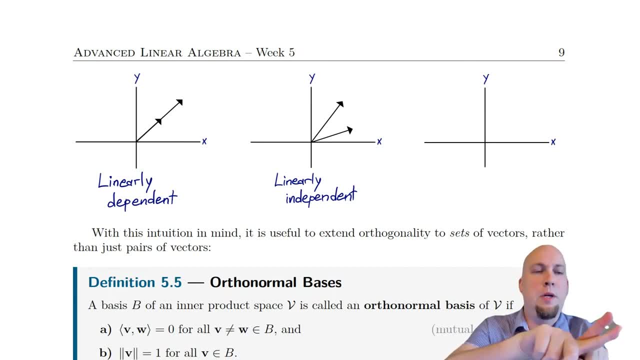 it's just the stronger version of this. not only are they not pointing in the same direction, but they're sort of pointing as far away from each other as they could before you start rotating back towards the span of each other. remember, the span of one of the vectors is the entire line in. 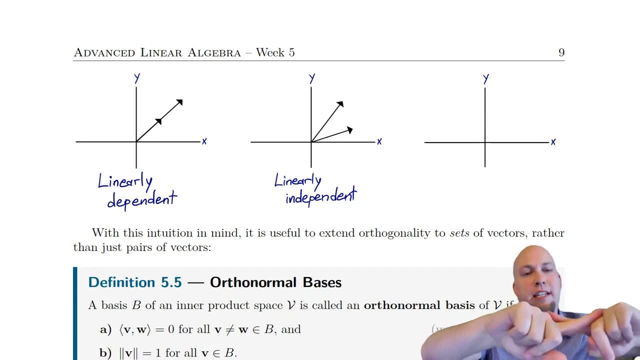 the direction of that vector. so once you go past pi over 2 or 90 degrees you start going back towards that same line. so orthogonality is sort of they're pointing in sort of as as not the same directions as possible. so that's our orthogonality picture. it's like linear independence. 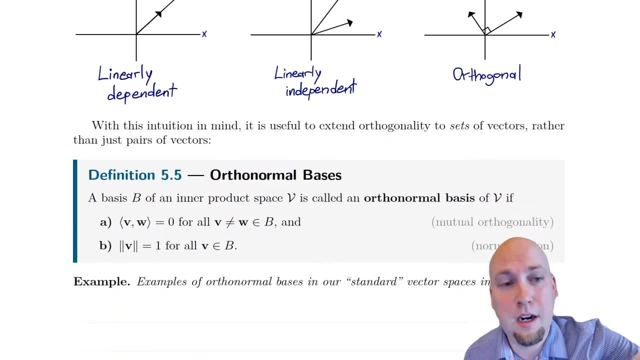 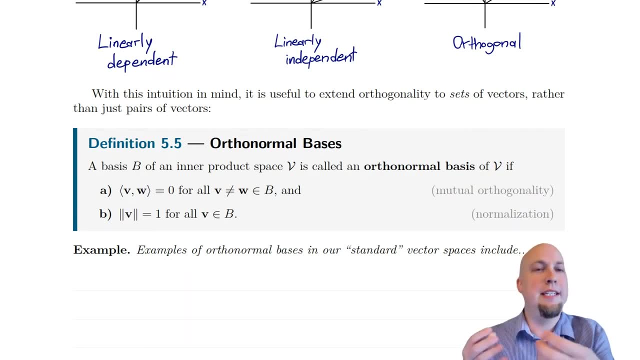 so that's our orthogonality picture. it's like linear independence, but on steroids, All right. So because linear independence is one of the main ingredients in bases, well, now that we have linear independence on steroids, it makes sense to ask the question. 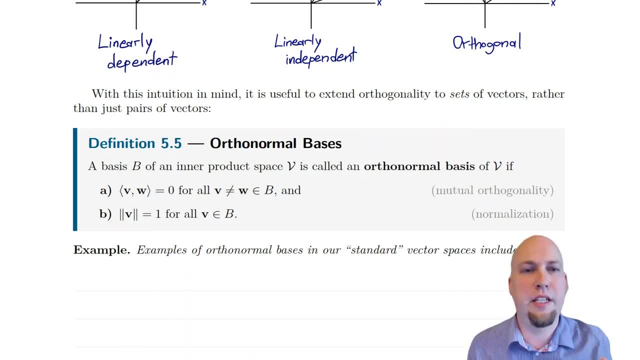 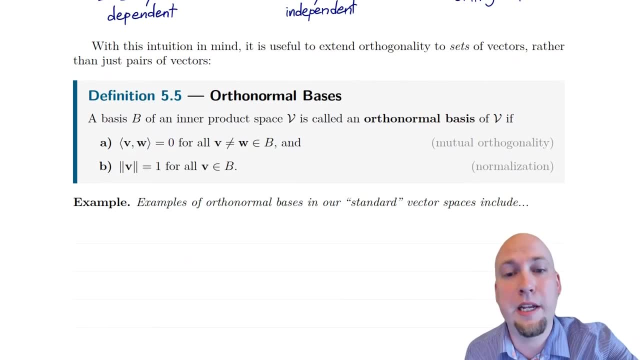 well, what happens to bases if you have this stronger notion of linear independence? What happens to bases if you have orthogonality instead? All right, So that's sort of our next step here. Now that we understand orthogonality, let's think about, well, bases where you have. 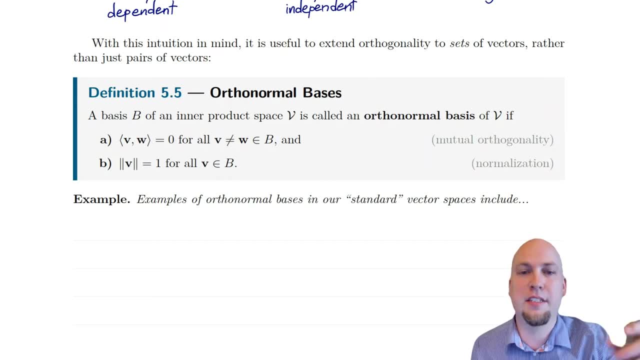 this orthogonality requirement rather than just linear independence, And we call these bases orthogonal bases, And we throw in one other minor condition: that we get something called orthonormal bases. So that's really the thing that we're going to be interested in, All right, So 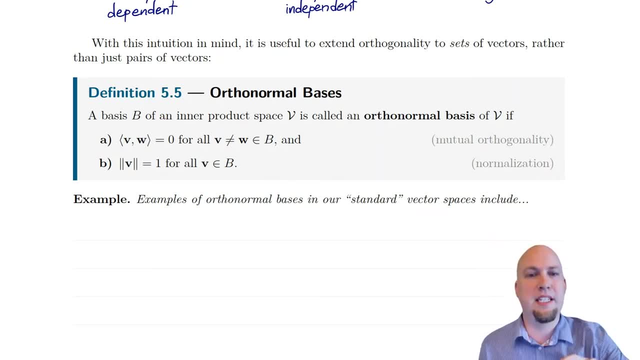 here's the setup. Suppose that you've got any old basis of an inner product space V, Okay, Well, we say that it's an orthonormal basis. if it has some extra conditions, Okay. The first extra condition is what we call mutual orthogonality, And it just means that every vector in that basis 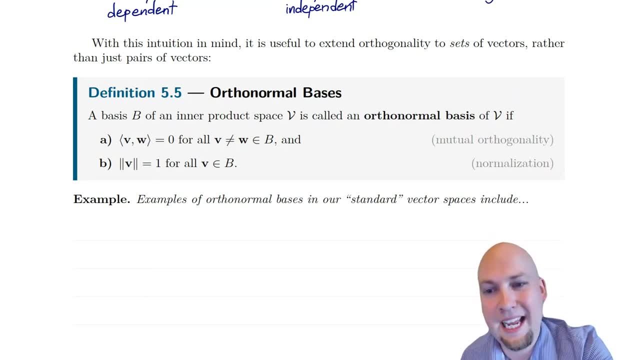 is orthogonal to everything. So if you pick any two vectors, V and W, the inner product equals zero. They're all orthogonal to each other. They're all sort of as independent from each other as possible. All right, And the other thing that we require is what makes it an orthonormal basis rather than just an orthogonal. 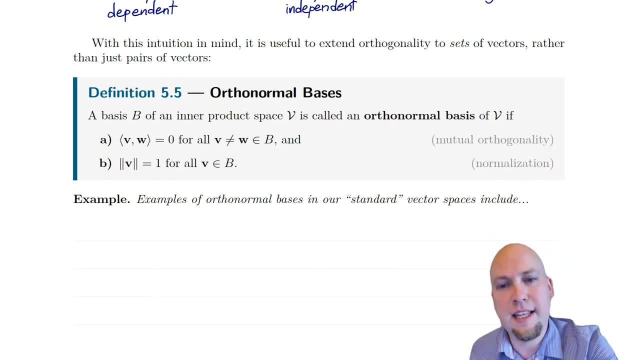 basis. Okay, So this normalization condition is just that we scale every vector in the basis to have length one, with respect to whatever inner product we're talking about. Okay, So this is sort of an easy condition to throw in after the fact, Because once you have an orthogonal basis, well you can just rescale everything to have length one. 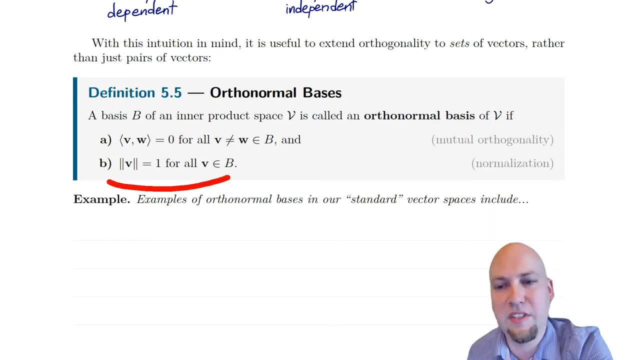 but by dividing every member of the basis by its length. So this is just sort of an easy extra condition that makes the basis even more well behaved. So we usually throw it in All right, And we have all sorts of standard examples of orthonormal bases in vector spaces that we've 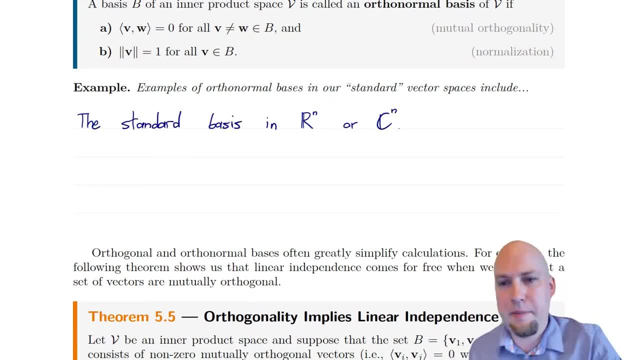 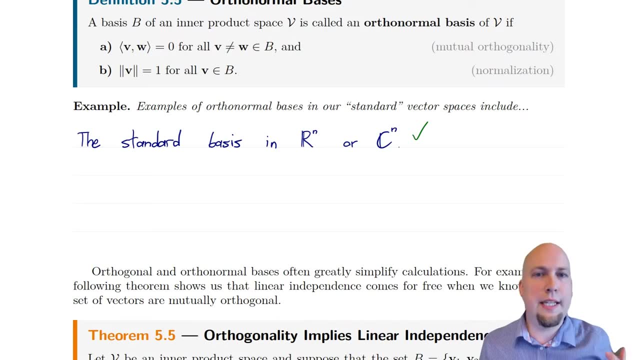 been looking at throughout this course. So, for example, I mean the standard basis in Rn or Cn. it's a straightforward calculation to show that, yeah, those really are orthonormal bases. Okay, I mean you have to check two things. You have to check this inner product. 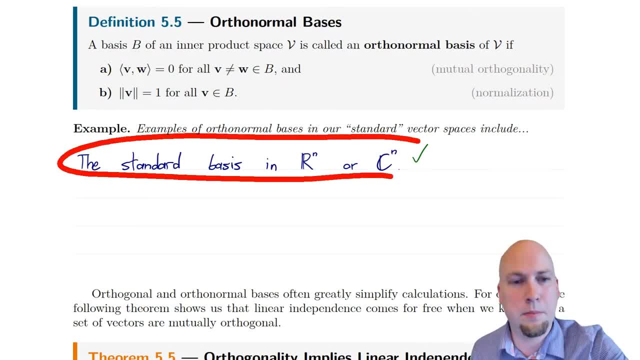 condition. Okay, And here I mean I'm just working with the standard inner product on these two spaces over here. So just the dot product. So these Ej vectors, right, these vectors that have one and a single entry and zeros everywhere else, If you take the inner product, the dot product of 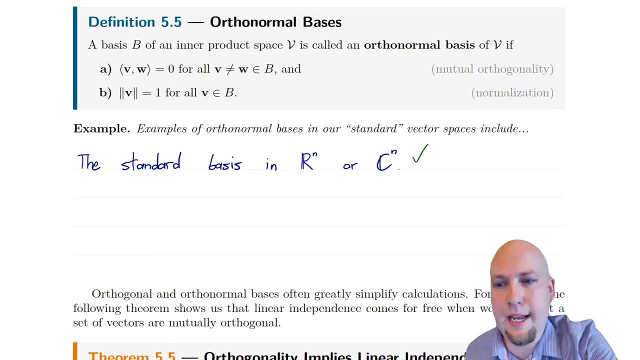 any two of those, you just get a bunch of zeros being added up. So, yeah, all of their dot products, all of their inner products are zero, Okay. And similarly, they all have length one. Again, that's straightforward to check. All right, If we go to our more. 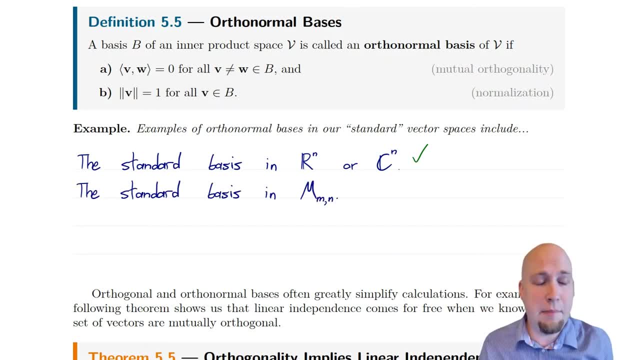 exotic vector spaces, like the space of M by N matrices. well, we've seen a standard basis in that vector space as well. Again, these are the matrices that have a one and a single entry and zeros everywhere else. And again, you just go through the calculation, use the standard inner. 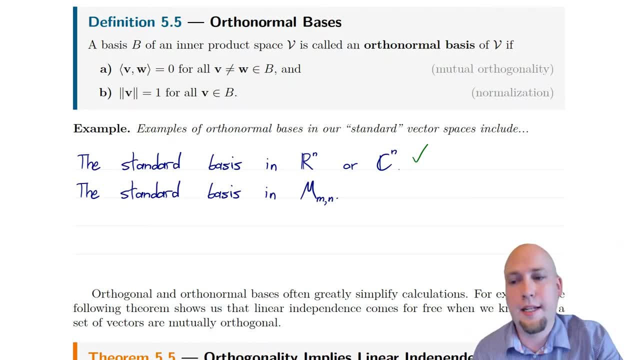 product, the Frobenius inner product, on this vector space. And it's just straightforward to check that. yeah, all of the inner products of those Eij matrices, they all equal zero and their lengths in the Frobenius norm, the norm induced by the inner product, those all equal one. 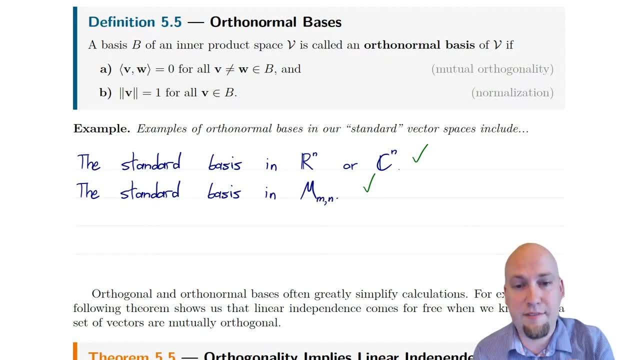 So yeah, that is an orthonormal basis in that vector space as well. And then, sort of continuing the trend, it seems natural to ask: okay, what about in the vector space PP, which, remember this is the degree less than or equal to P polynomials. And now on the real interval from: 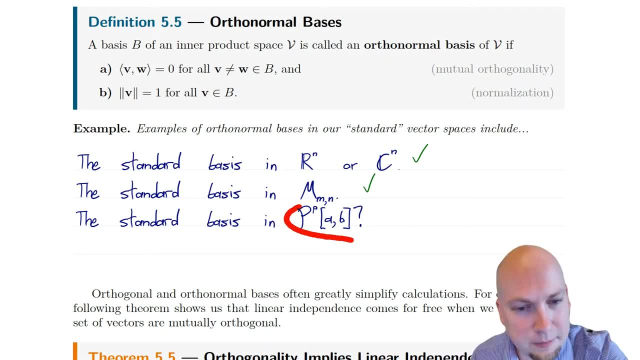 A to B. Okay, So what I mean by this is I'm working in the inner product space of degree P polynomials And the inner product I'm using is just the integral from A to B of this. you know, F of X times G of X, that standard inner product. 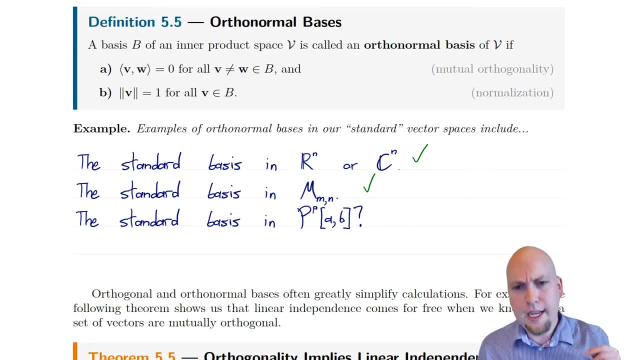 All right. And then the question is: well, is that an orthonormal basis? And this time we actually sort of break the trend a little bit. This is not an orthonormal basis. So you have to be a little bit careful when working in these function spaces. Okay, There are orthonormal bases in these function. 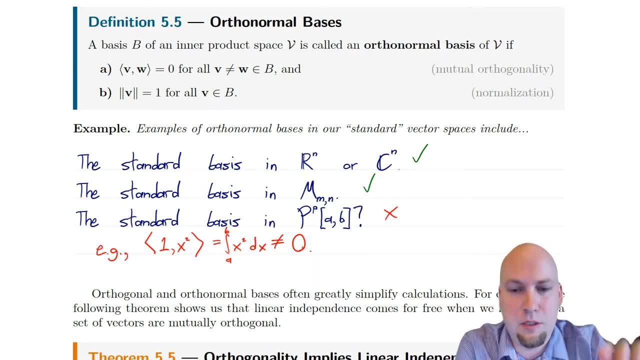 spaces, but they're actually all sort of uglier And we'll come back to this problem at the end of the week. All right, But to see that this is not an orthonormal basis in this vector space, let's just compute some inner products of some members of the standard basis. So, for example: 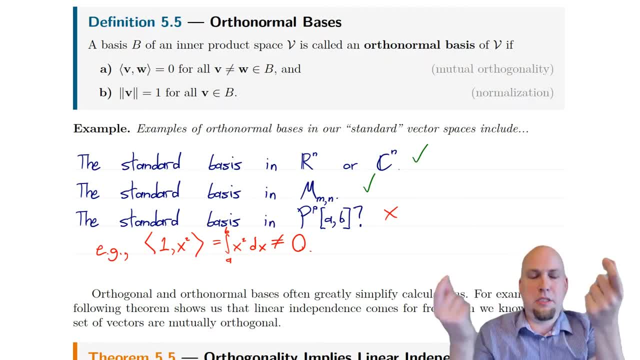 one and X squared. well, the inner product of that, you just multiply those two functions together, So you get X squared, and then you integrate from A to B, And because you're integrating a non-negative function- actually a strictly positive function, as long as you know- 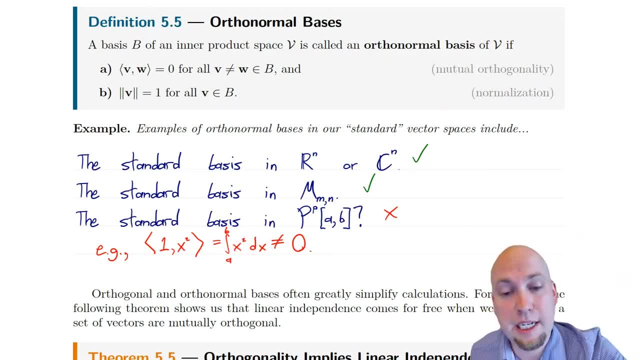 X is not zero. this integral is not going to equal zero unless A equals B, which you know not really a space to begin with. So this integral here is not going to equal zero, It's going to be something strictly positive, All right. So no, they're not orthogonal. 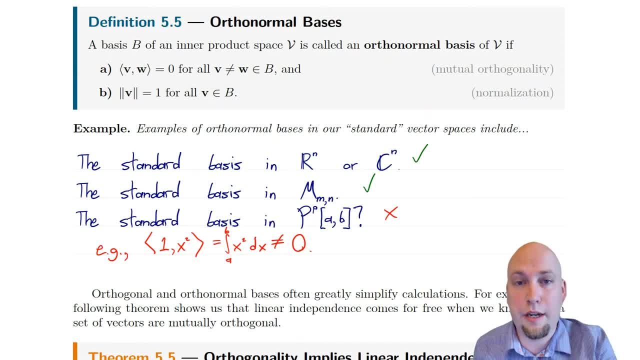 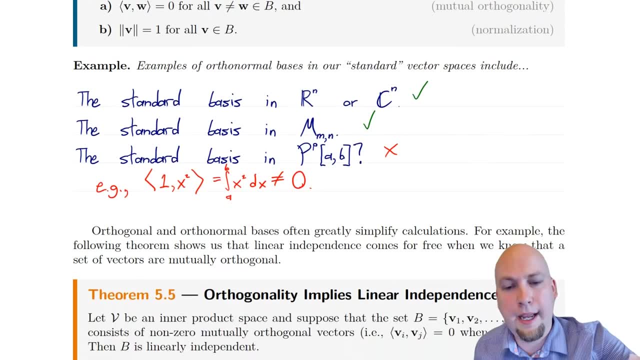 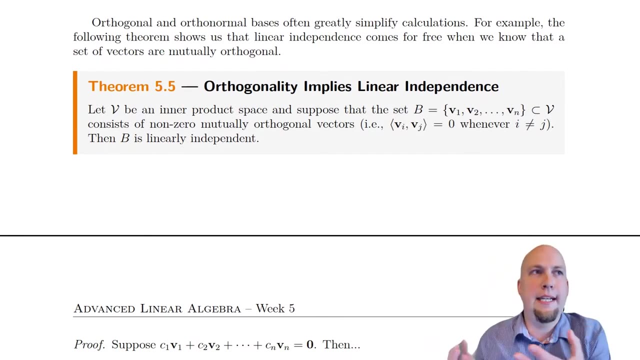 Okay, So that is not an orthonormal basis on that vector space. Well, we'll see an example of an orthonormal basis a bit later, Okay, Well, let's try to pin down this idea that we talked about earlier. We talked about how the idea behind orthogonality is sort of it's a stronger version. 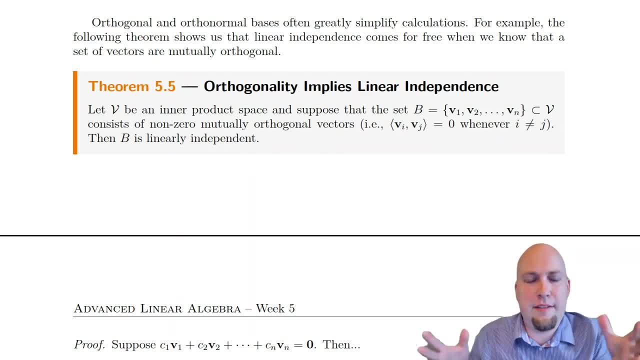 of linear independence. Let's pin that down. I mean sort of we have the geometric picture that sort of suggests it, but how do you prove it in an arbitrary inner product space? All right, So here's our theorem that pins down the idea that we talked about earlier. So let's see if we can. 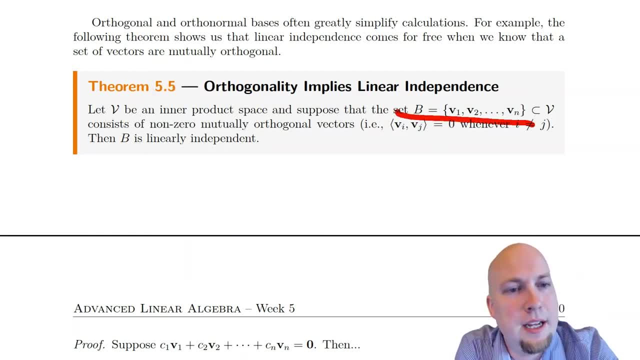 that idea. Suppose that you've got some inner product space. and suppose that you've got some set B that consists of non-zero, mutually orthogonal vectors- Okay, So the idea here is, you've got something that sort of looks like an orthogonal basis. Okay, So all of the vectors have to be. 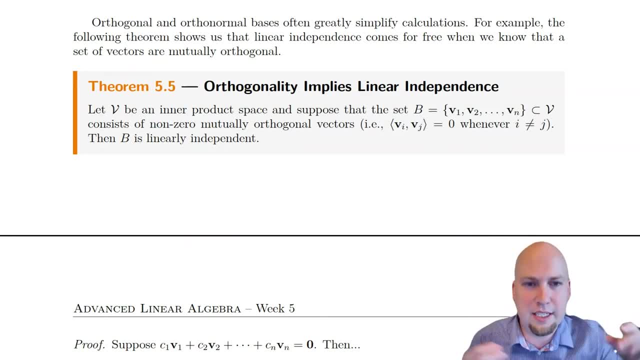 non-zero just because, well, I mean, the zero vectors are orthogonal to everything, So we sort of need to take away that trivial case And then mutually orthogonal again. just remember what that means is that they're all orthogonal to each other. You take the inner product of any two of 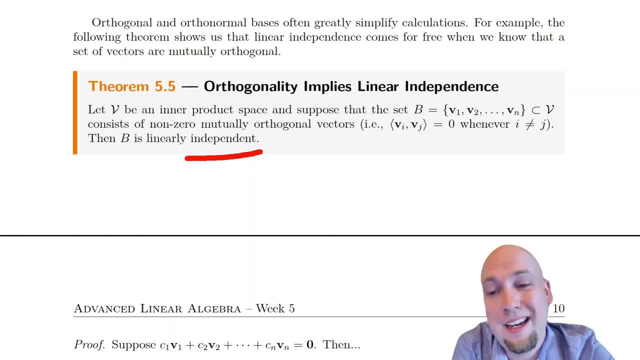 them. So if you have a set like that, where all the vectors are orthogonal to each other, then it must be linearly independent, All right. So let's pin down this idea. Let's see why orthogonality implies independence. All right. So the setup here: we want to show that some sets linearly. 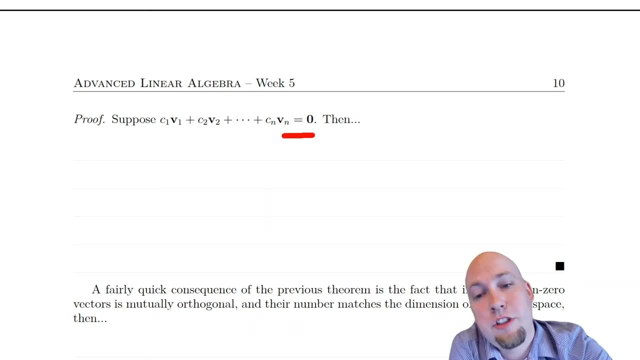 independent. The way you do that, remember, is you show that the only solution of this linear system here is the all zero solution. So in other words, you show that this linear combination equaling zero implies that all of the C's have to equal zero. So that's what we're trying to do. 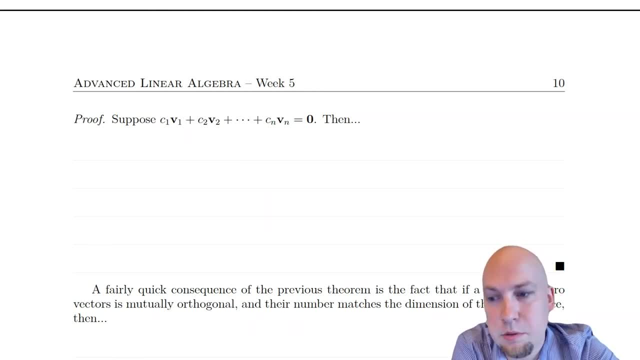 We're going to try to do here. We're going to try to show that each of the C's has to equal zero, All right. So the way we do- that is what we're going to do- is we're going to take this linear. 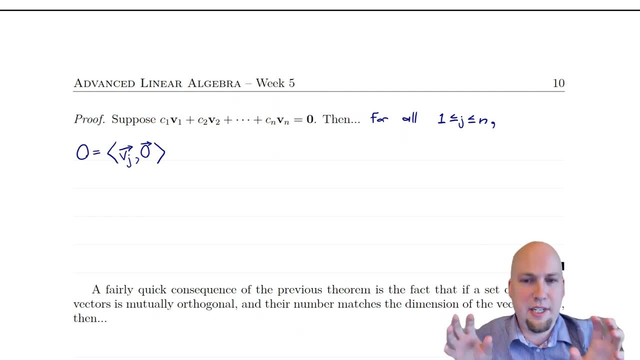 combination here and I'm going to take the inner product of it with the vector vj, with the jth vector, from the basis. Okay, I'm going to do that both on the left-hand side and on the right-hand side, And I better get the same thing when I do that. All right, Well, starting off on the right-hand, 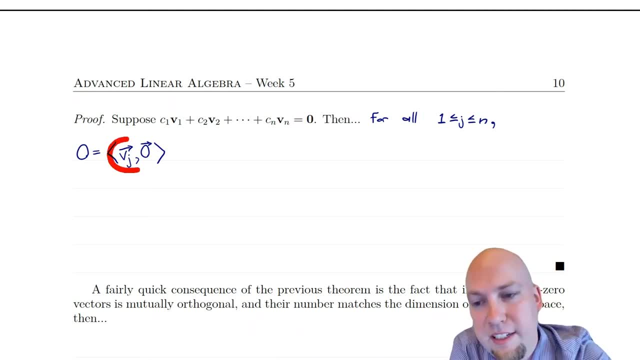 side. if I take the inner product on the right-hand side with the vector vj, well, it's just some vector inner product with a zero vector. I'm going to get zero, Okay. On the other hand, if I do the same inner product on the left-hand side with vj, what do I get? Well, now I get this junk. 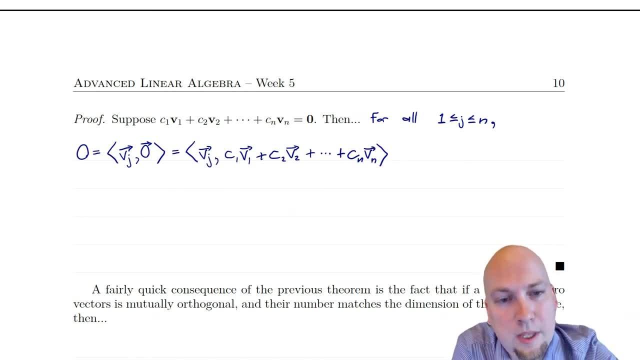 over here. Okay, I get vj inner product with that linear combination, right, I just substitute out: zero equals that linear combination, And now I'm going to use properties of inner products to sort of break that apart and simplify it as much as I can. Okay, So linearity in the second entry of 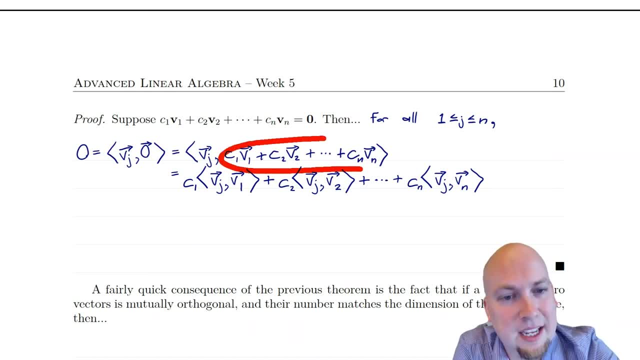 the inner product tells me that I can split it apart like this: I've just split this linear combination up outside, So now it's just c1, v1 with vj, c2, v2 with vj, and so on down the line. All right, Next up. 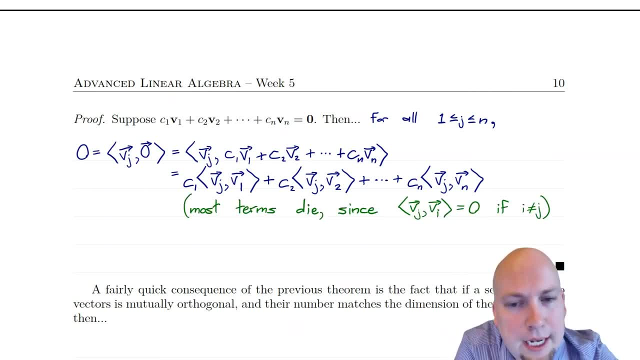 Now I'm going to notice that hey, over on the right here. what I've got is I've got the inner product of two vectors in that set B And I've got the inner product of two vectors in that set B and then the inner product of two vectors in that set B, But B it's a mutually orthogonal set. 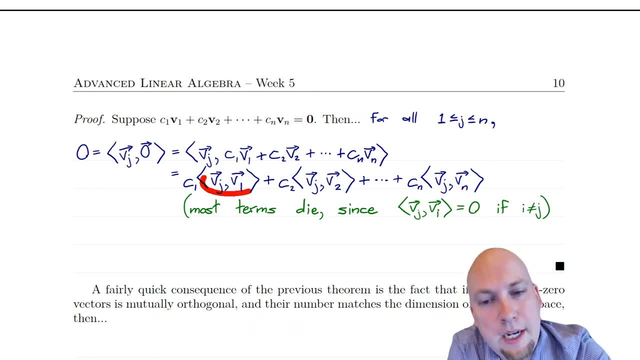 So all of these inner products actually equal zero, right? Because all except for one. okay, right, Because every vector in the set is orthogonal to every other vector in the set. So the only term in this sum that does not die is the one where it's vj inner product with vj. 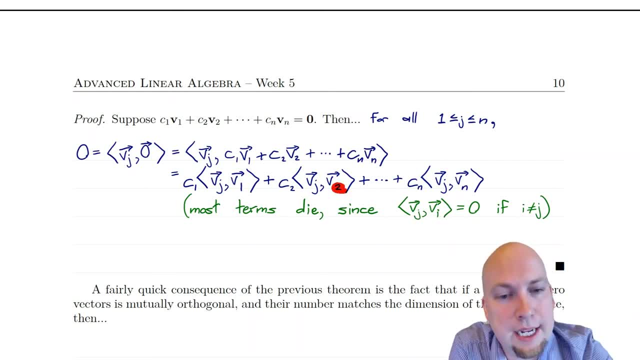 Okay, So most of these terms die. Whenever the subscript over here on the right is not j, the term goes away. That inner product is zero. Okay, So all I end up with out of this sum is the term cj times vj: inner product with vj. All right Now, because this all equals zero. 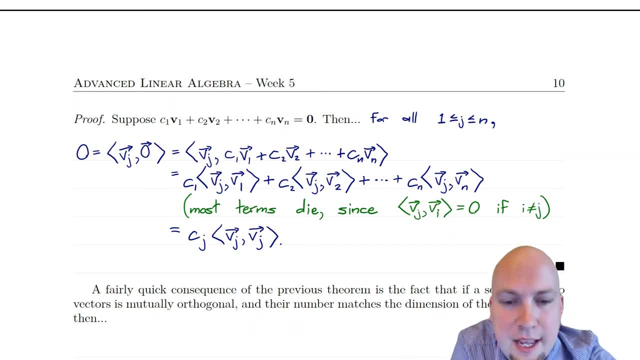 right. If I trace this through, this equals zero. Well, now I look at this. Can this inner product over here equals zero? And no, it can't, Because if you go back and look at the defining properties of an inner product, 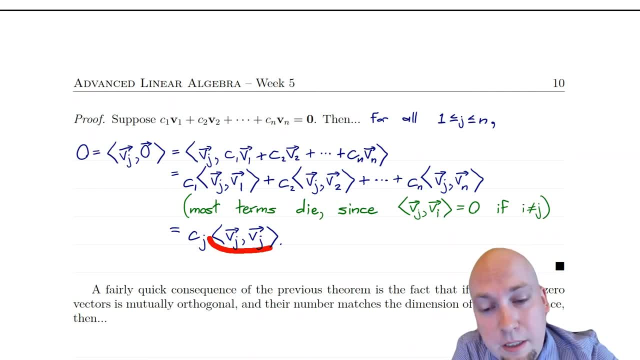 the third defining property was: whenever you take a vector and inner product with itself, you get something bigger than or equal to zero. And furthermore, the only way to get zero is if the vector is the zero vector. But go back to the statement of the theorem We're 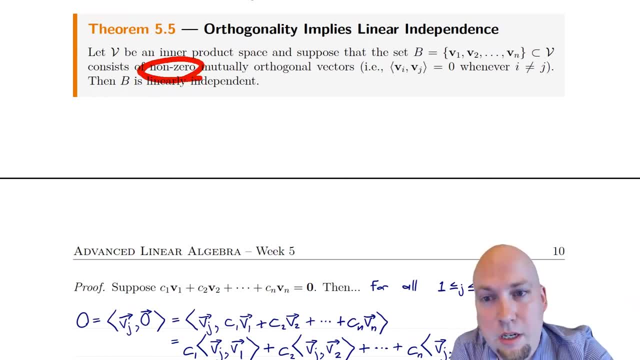 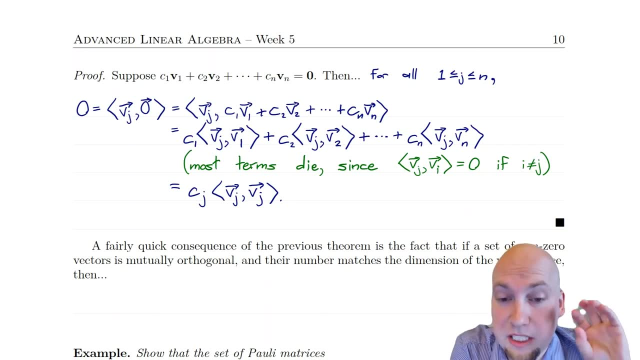 assuming that every vector in the set B is non-zero, It's not the zero vector, Okay. So this inner product over here cannot equal zero. In fact it's got to be strictly bigger than zero. So the only way that this product here can equal zero is if cj itself equals zero. So yeah, 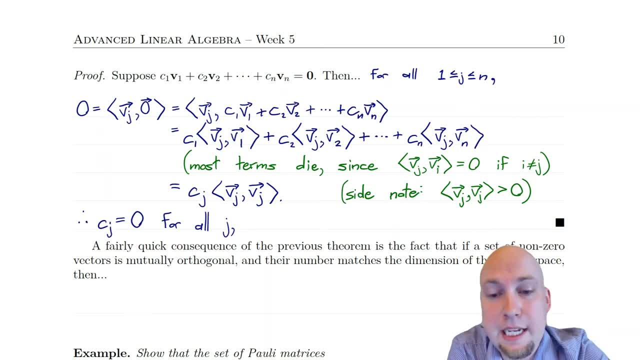 that inner product is bigger than zero. So therefore cj equals zero. for all j right, Because it didn't matter what j was. So in other words, we got exactly what we wanted. We got that each of these coefficients here equals zero. All right, So B must be a linearly independent set. 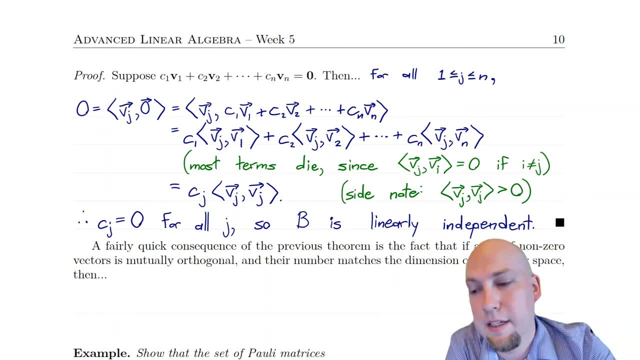 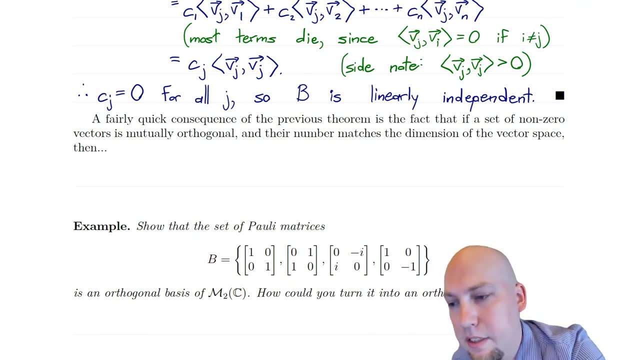 So yeah, mutual orthogonality does imply linear independence. Okay, If we combine this with earlier results we saw earlier in the course, a fairly quick, really nice corollary of this is that if you have any set that is A mutually orthogonal 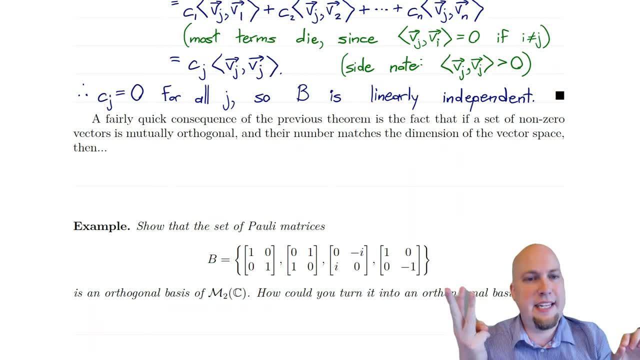 B, all of the vectors are non-zero and, C, the number of vectors in that set matches the dimension of the vector space that they live in, then you know right away that they must form an orthogonal basis of that space. Okay, Because that means that if you have a set that is a, 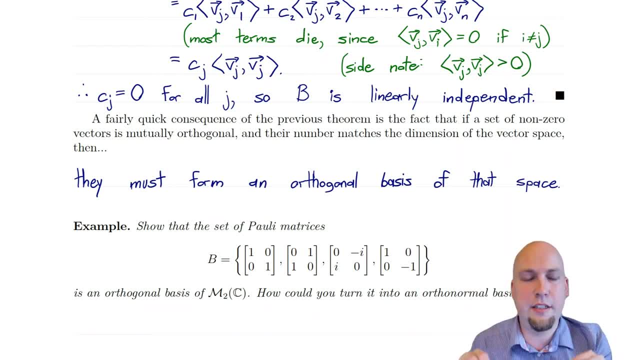 non-zero, then you can have a set that is a non-zero and that's a non-zero and that's a non-zero. So mutual orthogonality and non-zeroness implies that they're linearly independent, And then the fact that their dimension matches up with the space implies that they span the entire. 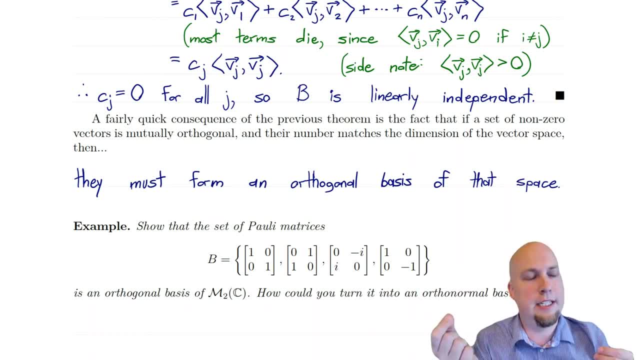 space. right, We have this theorem that tells us that if you have linear independence and the dimension and the size of the vector is the dimension of the space, then actually it's a basis Okay. So in a sense you're getting both spanning and linear independence almost for free. 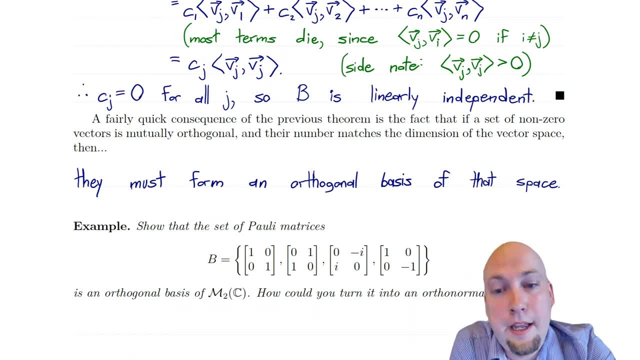 now. Now, all we have to do to check whether or not something's an orthogonal basis of a vector space is just check orthogonality and then count All right, So it becomes really, really easy. We got a lot of stuff for free here, So let's do an. 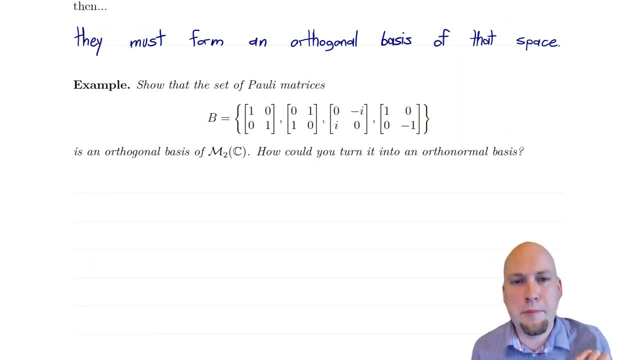 example here of showing that something is an orthonormal basis, or at least an orthogonal basis, of a vector space, And what we're going to do is we're going to show that this set of polymatrices that we've seen a couple of times now, let's show that this really is an orthogonal. 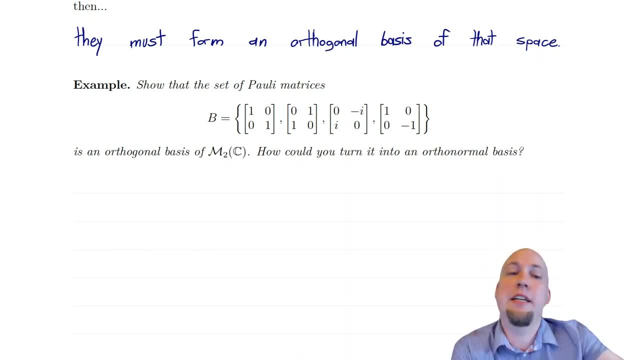 basis of the space of two by two complex numbers. We've seen earlier that this is a basis of that space, And the way we did that, we had to solve a bunch of linear systems to show linear independence and spanning. Now we'll show this property without solving any linear systems at all. Okay, So how do we do this? 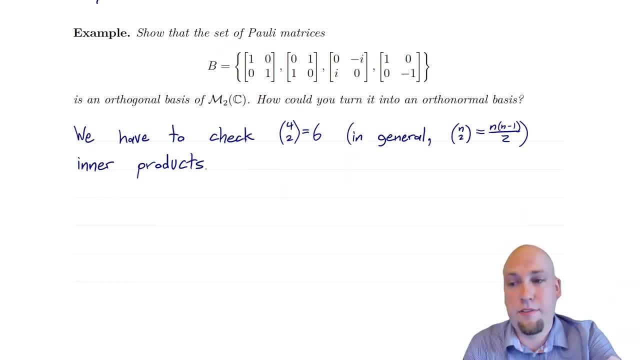 Well, we've just got to compute a whole bunch of inner products, right? So first off, we note, I guess, that Hey, there's four vectors here, right? And I already know that M2 of C, that's four dimensional. So I have the right number of vectors, right number of matrices. I just need 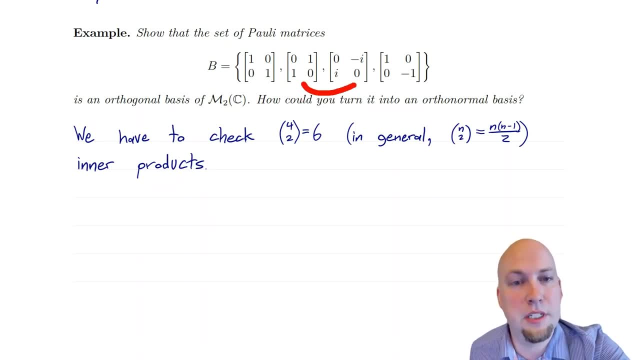 to check whether or not the inner products of all these pairs equals zero, right, So that you have to check six different inner products here, because how many pairs are there of four matrices? Well, there's six of them, It's four. choose two. In general, if you have a vector space, that's N. 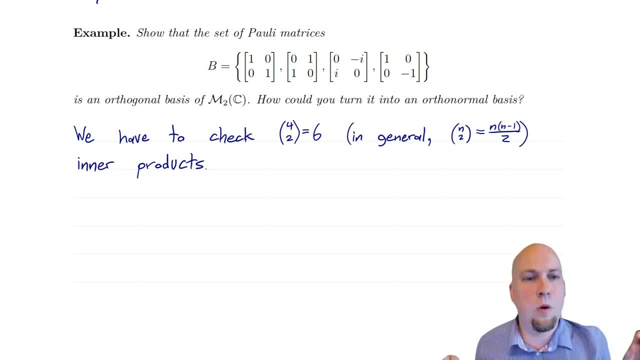 dimensional. so you have N vectors that you need to check orthogonality between them. you have to do N, choose two pairs. So N times N minus one over two, with that many inner products that you have to check. All right, So let's just check all of these inner products. I'm not actually going to. 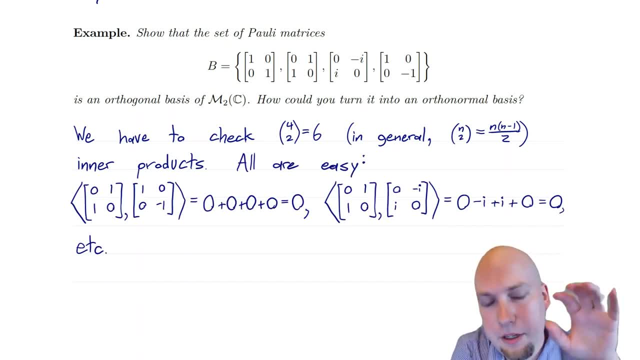 go through all six of them. They're all just straightforward, right? You use the standard inner product here because, again, I haven't indicated otherwise. So we're just using the standard Frobenius inner product, All right, And let's just check some of these inner products. So here I took 0, 1, 1, 0.. So this: 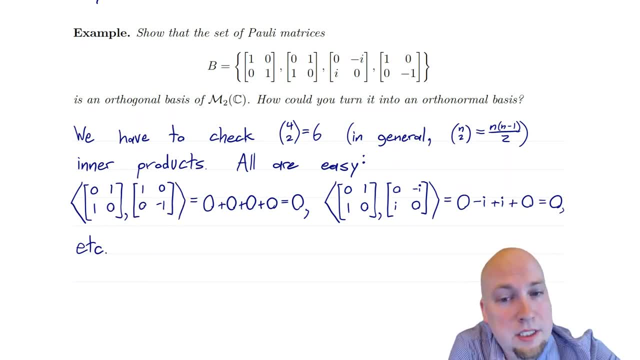 basis matrix and I took the inner product with 1, 0,, 0, minus one, So this one here. So I did this pair And remember the way the Frobenius inner product works, you could use that trace formula or you could do: hey, just multiply them entry-wise and add them up, right, It's the dot. 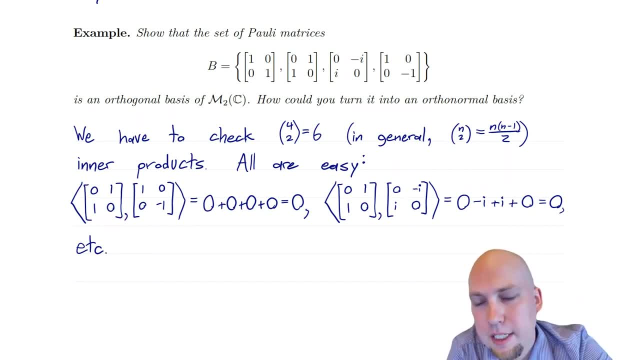 product for matrices, And you have to be careful. throw complex conjugates on the first matrix, but they're all real here, So it doesn't make a difference. So you just do: zero times one: Ah, that's zero. One times zero, That's zero. One times zero: Ah, that's zero. Zero times minus one: Ah, that's. 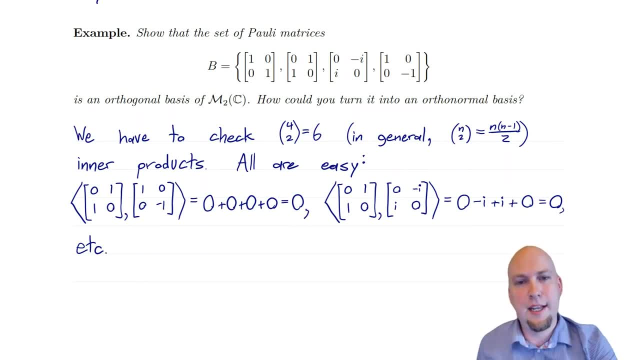 zero. Add them up. I'm adding up four zeros, I get a zero. Okay, So yes, this pair here they're orthogonal to each other. Let's do another one. Okay, Let's do this matrix with this matrix. Okay, 0, 1, 1, 0 with zero minus I, I zero Again, just do it entry-wise: Zero times. 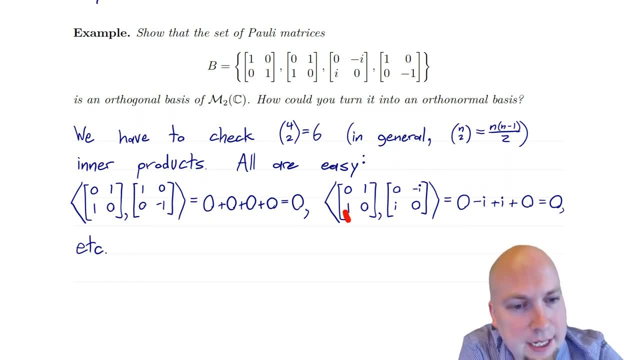 zero- Ah, that's zero. One times minus I: Ah, that's minus I One times I. That's I. Zero times zero- Ah, that's zero. Add them up: Ah, of course, You get zero. Okay, So they're orthogonal to each other as well. There are four. 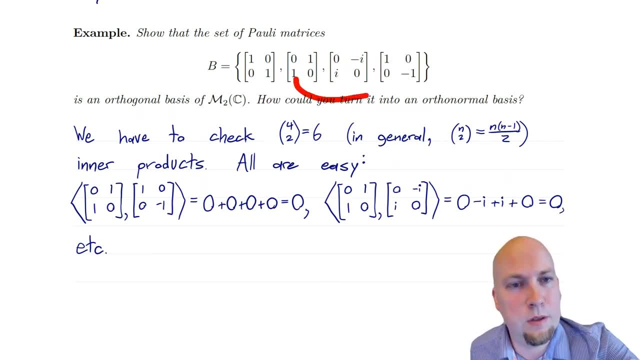 other pairs that we haven't done, but you can just check those straightforwardly yourself. I mean, they're all just as easy to do as these two here. Okay, So now that you've checked orthogonality, great, We know that it's an orthogonal basis of the space of two by two complex matrices. 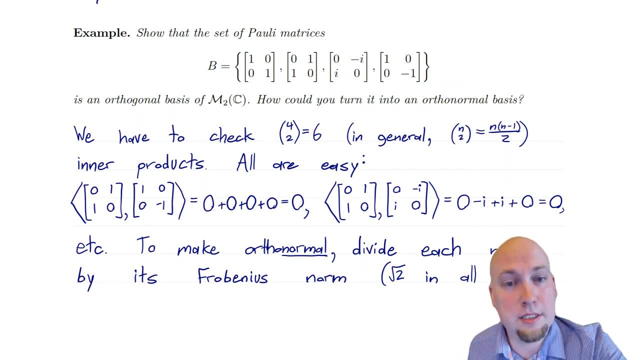 To make it an orthonormal basis, right. The question also asks: how can you turn it into an orthonormal basis? Well, to do that, just take every vector, every matrix in that set and divide it by its norm right, Divide it by the norm induced by whatever. 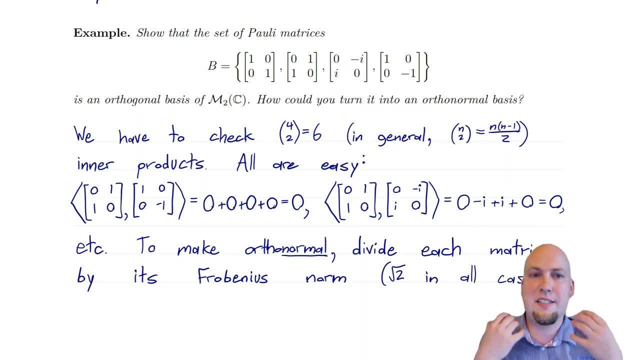 inner product you're working with. Okay, So again, here we're working with the standard inner product, the Frobenius inner product. So just compute the norm with respect to the Frobenius inner product of each of these matrices. here It's going to turn out that each of these